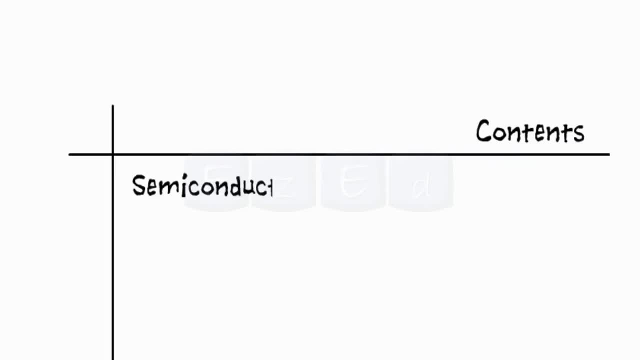 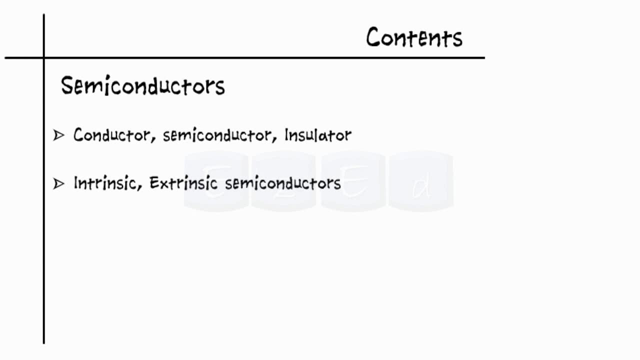 In this EasyEd video lecture, we're going to learn what are conductors, insulators, semiconductors, the difference between intrinsic and extrinsic semiconductors, as well as P-type and N-type semiconductors. Now let's first understand the materials. 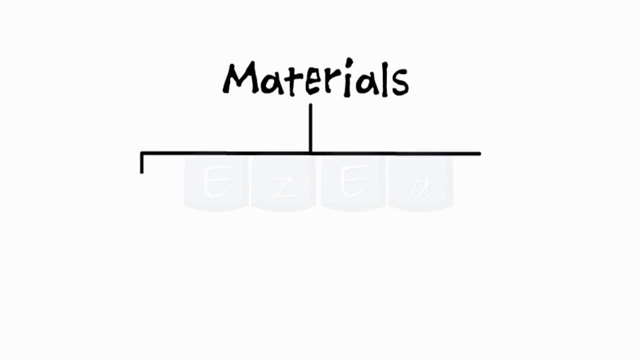 When we talk about materials in electronics, we compare them to their current carrying capacity, and they can be classified into three types, namely conductors, semiconductors and insulators. Conductors are materials that have excellent current carrying capacity or allow good flow of current through them, such as a copper wire. 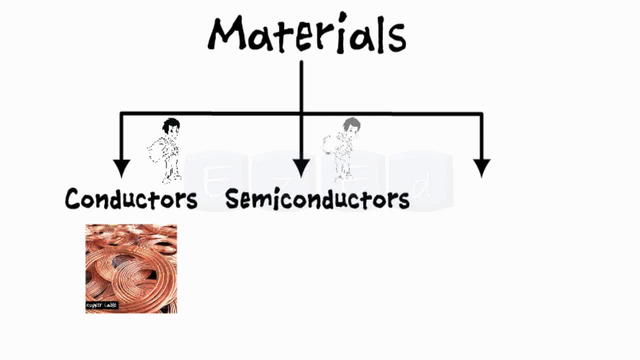 And semiconductors, as the name suggests, allows partial or semi-conduction of the current, or we could say its current carrying capacity is in between the conductor and the insulator, such that it can carry a lot of current, Such as germanium. 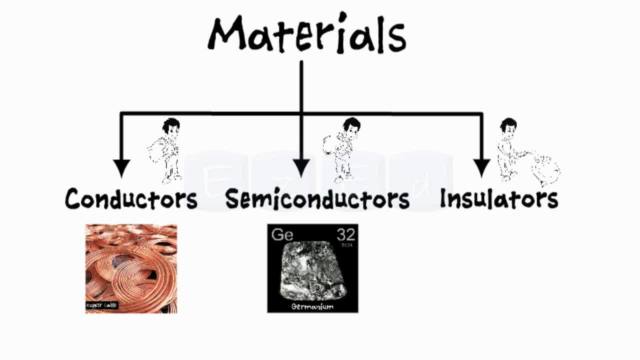 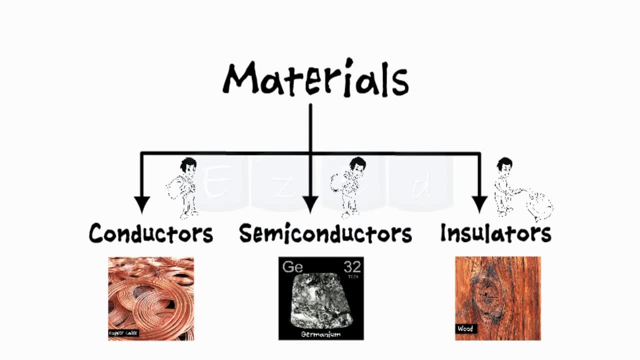 Whereas insulators are materials that are bad conductors of current and do not allow the flow of current through them as they do not have a current carrying capacity, such as wood. Now let's further understand this with an example of a stadium entrance and people. 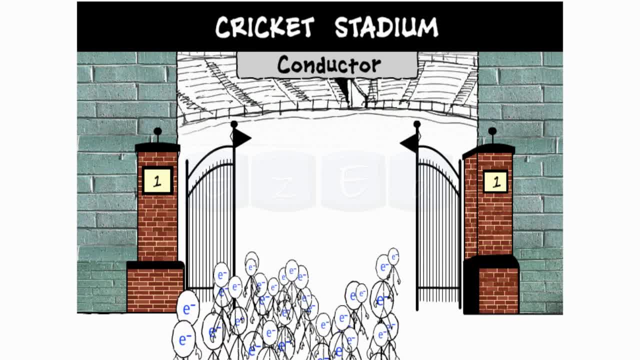 Let's imagine the stadium entrance to be a conductor and the people as current. Now we can see a large group of people passing through the gates and enter the stadium easily. in the same way, In the same manner in which conductors allow electricity to pass through them easily. 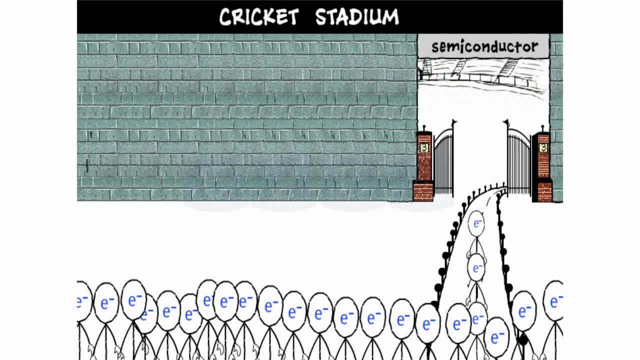 However, here we see the crowd of people moving past the entrance, one by one, slowly, in a queue. Now, why is that? That's because the current in a semiconductor passes through it partially, but continuously. In the case of insulators, that are bad conductors of electricity. 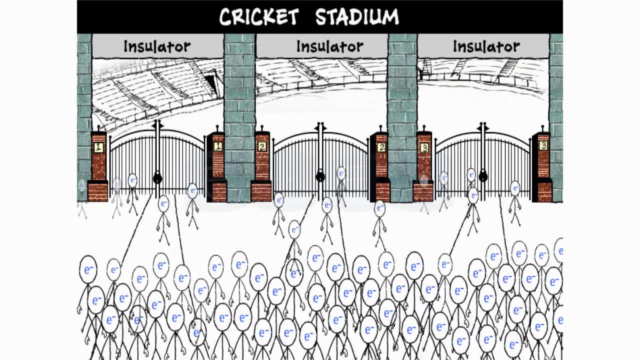 we can see, the stadium entrance, which we have assumed to be an insulator, is blocked, Thus not allowing the crowd of people which we have assumed to be as current to pass through it. The term semiconducting was used for the first time by Alessandro Volta in 1782.. 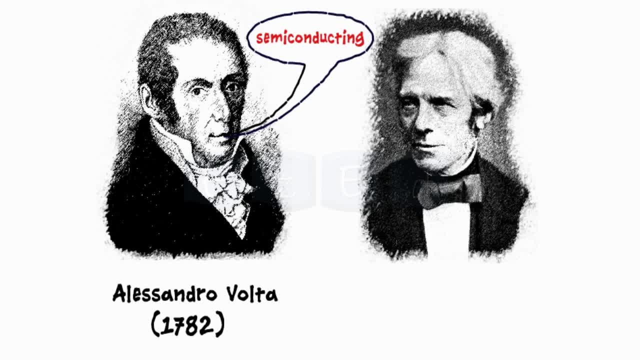 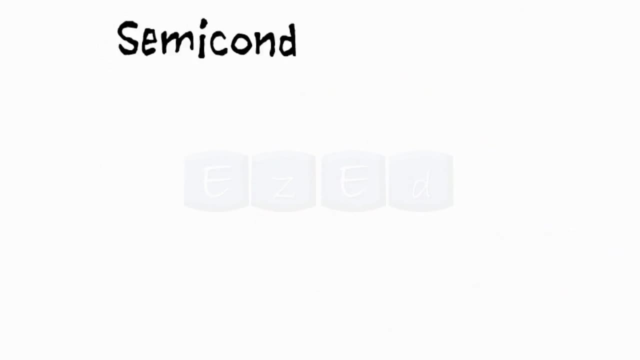 However, the first documented observation of a semiconductor effect is that of Michael Faraday in 1833, who noticed that the resistance of silver sulphide decreased with temperature, which was different than the temperature dependence observed in metals. Semiconductors are further divided into intrinsic and extrinsic semiconductors, depending on their structure, properties, etc. 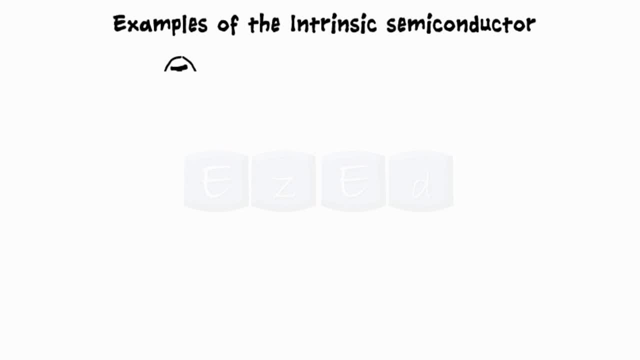 Intrinsic Semiconductors. Do we know what intrinsic means? It means in its purest form. Therefore, these types of semiconductors are in their purest form, by the nature of their existence. The common semiconductors used are silicon and germanium. 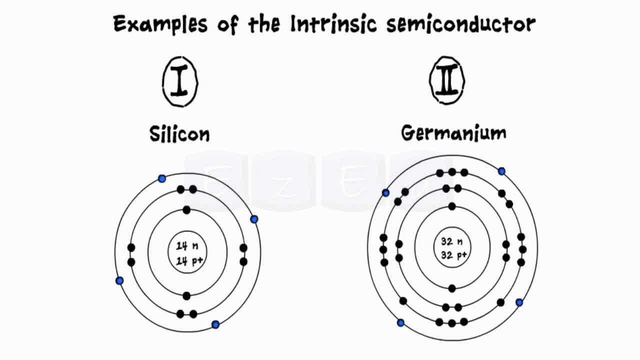 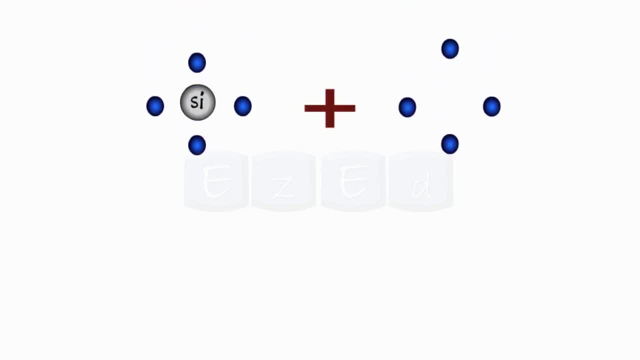 and they have four valence electrons orbiting in its outermost shell. We can further understand the motion of these electrons by looking at the structure of its atom. However, the atom needs a total of eight electrons in its outer shell to become stable. 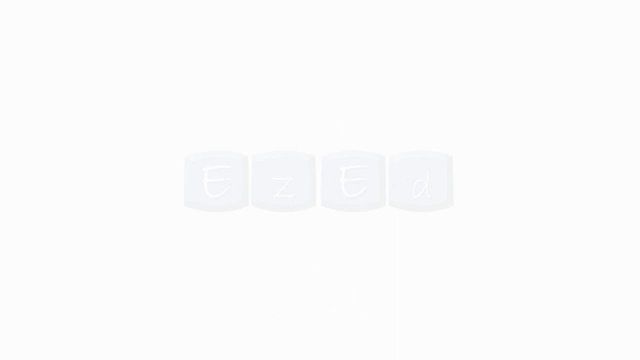 Hey, it's time to concentrate now. Now let's see how the semiconductor atom acquires the additional four electrons and becomes stable. Let's first look at this process with the help of one atom. It has its four valence electrons and requires an additional four to become stable. 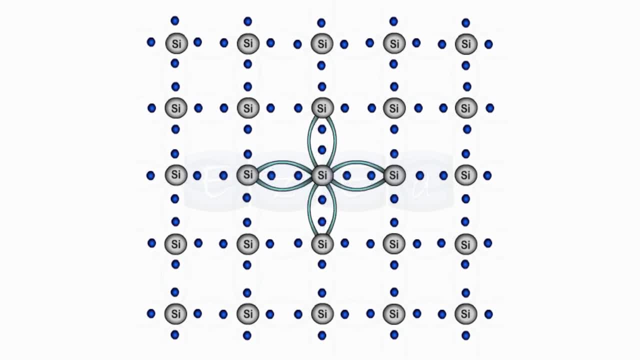 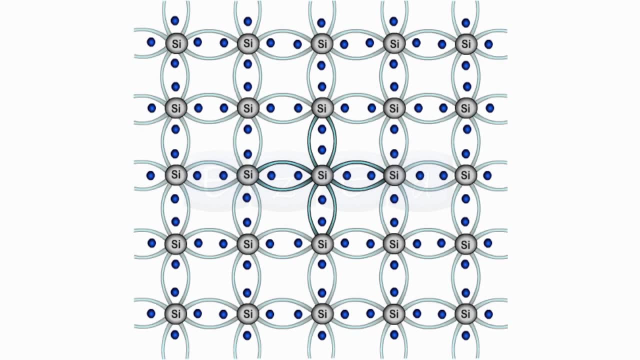 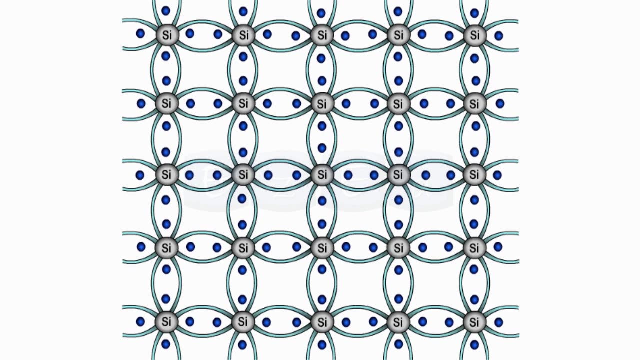 which it shares with its neighbouring atom, so that every silicon atom has eight electrons in its outermost shell. Here millions of silicon atoms are bonded together and they form a semiconductor structure which looks like this: All these atoms set up a bond with each other, which is called as a covalent bond. 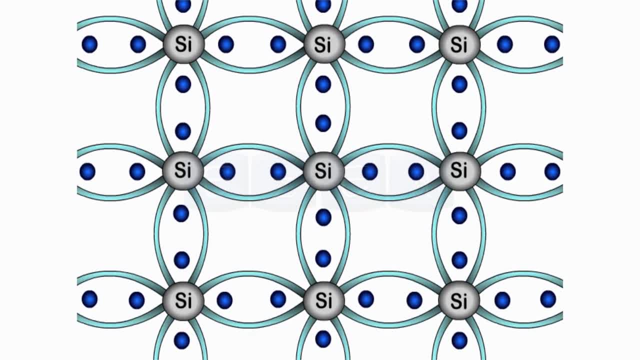 However, these bonds are so strong that the electron fails to break the bond at zero kelvin. But as the temperature increases, the electron absorbs the heat energy and it is able to break the bond. Once the bond is broken, the electron becomes free to carry the current. 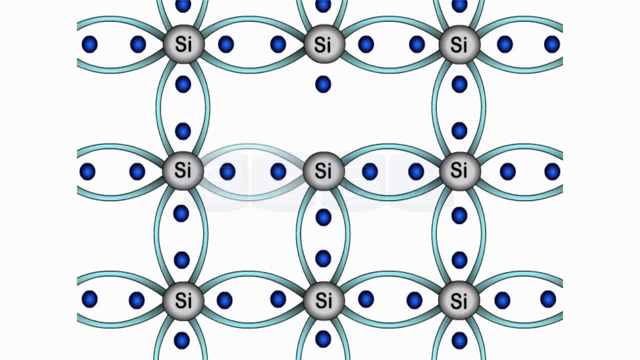 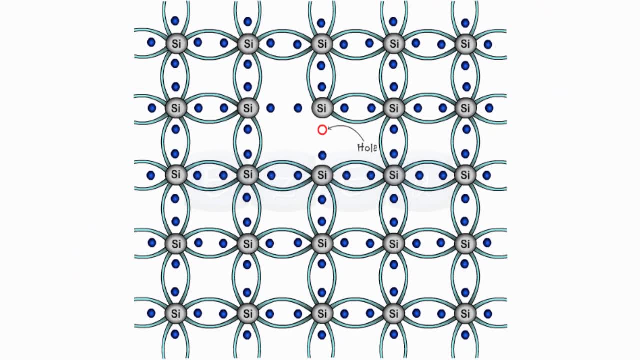 We get a deficiency of an electron in the structure. Hence there is an empty space formed, which can also refer to as a hole. Therefore we consider holes to be positively charged. Electron here is negative and the empty space or hole is positive. Therefore the immediate 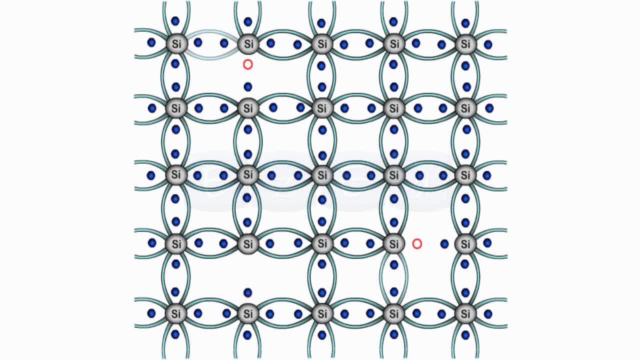 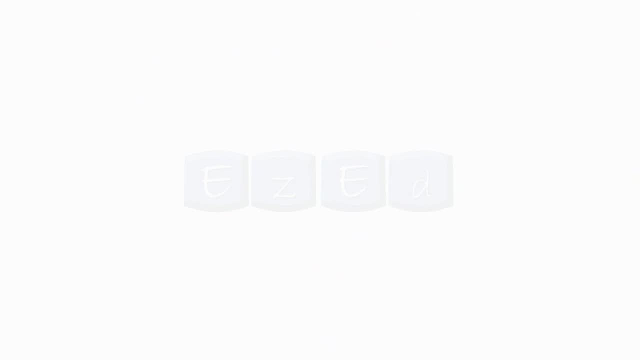 neighbouring electron gets attracted towards this hole and fills its place, thus creating another empty space or hole At its previous position. the process will continue in the entire structure in a random manner. So let's understand the second type of semiconductors, which are extrinsic semiconductors. 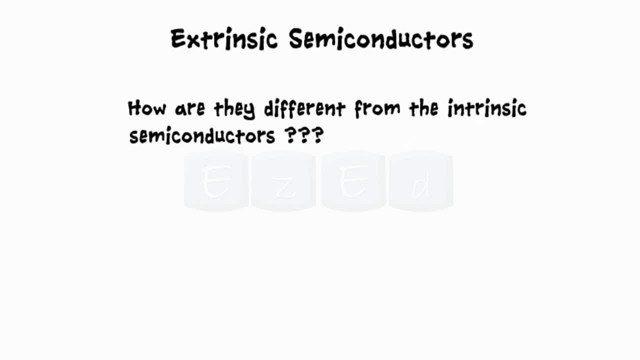 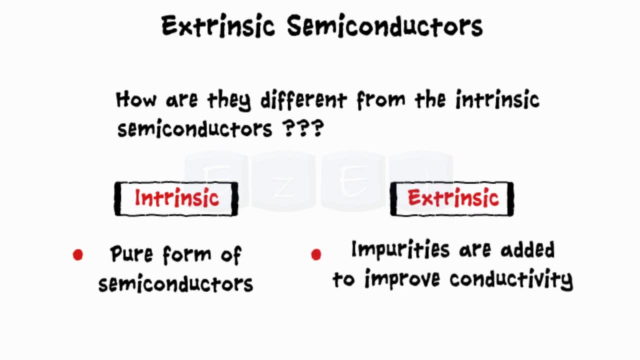 How are they different from the intrinsic semiconductors? While intrinsic are the pure form of semiconductors, impurities need to be added to the structure. These semiconductors need to be added to the intrinsic to improve their conductivity, and these semiconductors with impurities are called as extrinsic semiconductors. 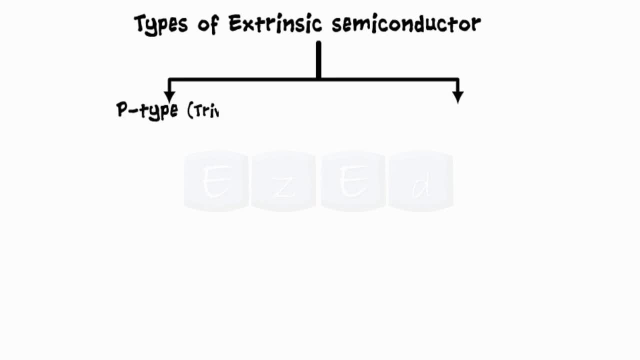 Extrinsic semiconductors are further subdivided into p-type or trivalent, and n-type or pentavalent. As we can see, we have three electrons orbiting in the outermost shell of the atom. It is called as trivalent. 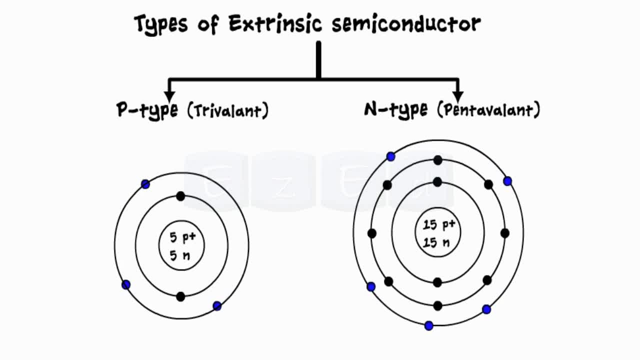 And in the other atom we have five electrons orbiting, Hence it is called as pentavalent. The common examples of trivalent are boron gas, potassium and indium, and that of pentavalent are phosphorus, arsenic and antimony. 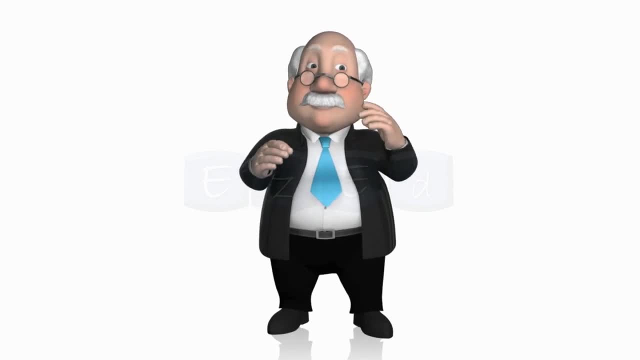 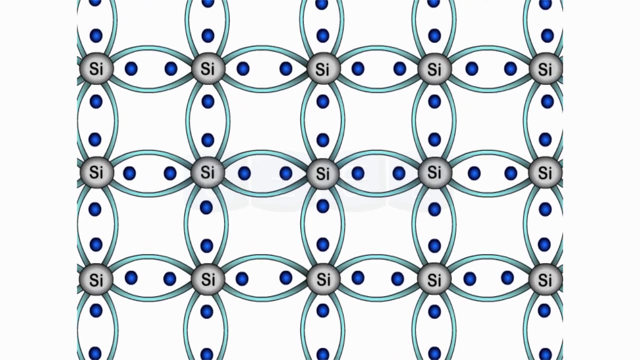 Seriously pay attention. This is important. The process of adding these impurities to the intrinsic semiconductors is called as doping, and the impurities that improve the conductivity of these semiconductors are called as dopants. In case of trivalent, three electrons of boron will form three bonds with silicon and in the fourth bond of silicon. 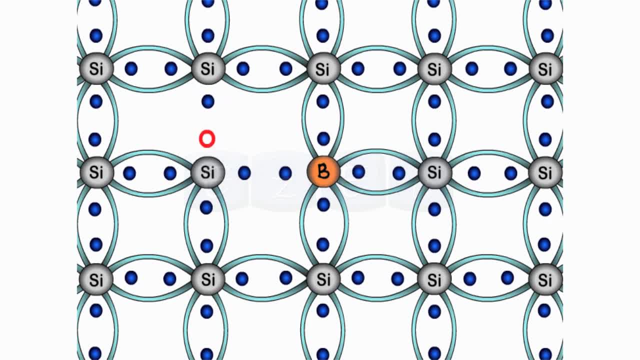 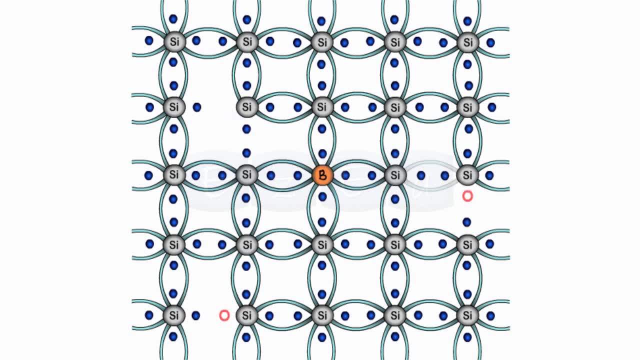 There will be one empty space or hole And, as seen previously, the immediate neighbouring electron will be attracted towards the hole, thus creating another empty space in its previous location. Simultaneously, the electrons of the silicon atoms attain thermal energy and keep breaking the covalent bonds at room temperature. 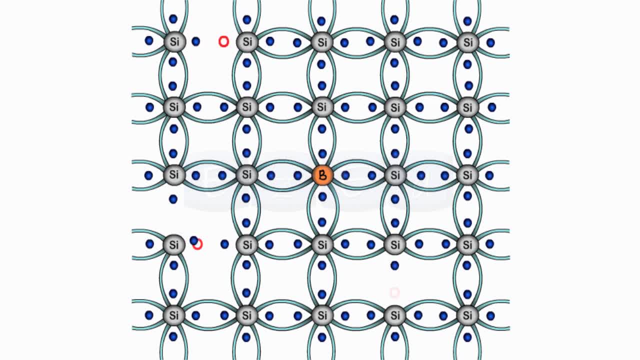 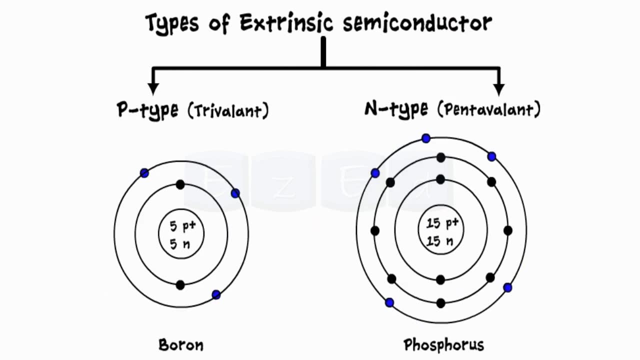 thus creating further free electrons, and this movement will go on in the same manner. Therefore, the number of holes generated in this structure dominate over the electrons. Hence this structure is called as a p-type semiconductor. Now let's look at the second type of extrinsic semiconductor, the n-type or pentavalent semiconductor. 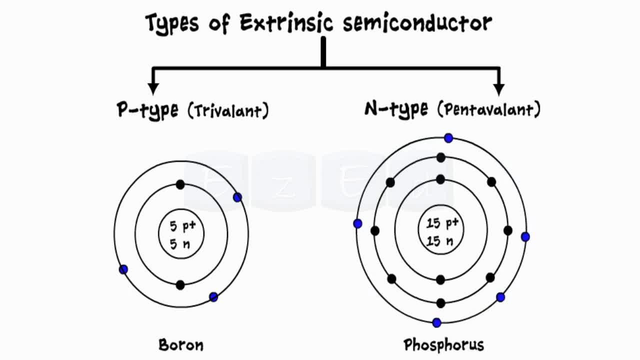 In this, the atomic structure of the n-type or pentavalent semiconductor will have five electrons in the outermost shell. As silicon requires only four additional electrons to attain stability in pentavalent atom, we have one extra electron as the valence electron. 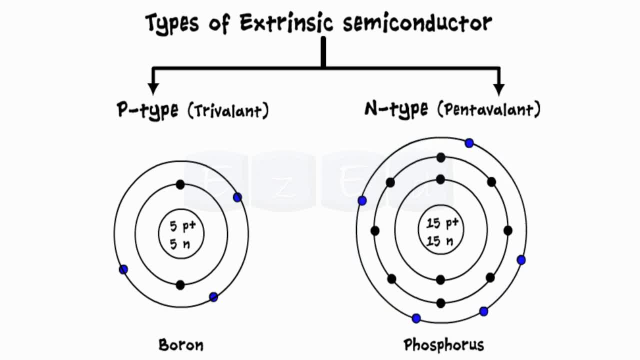 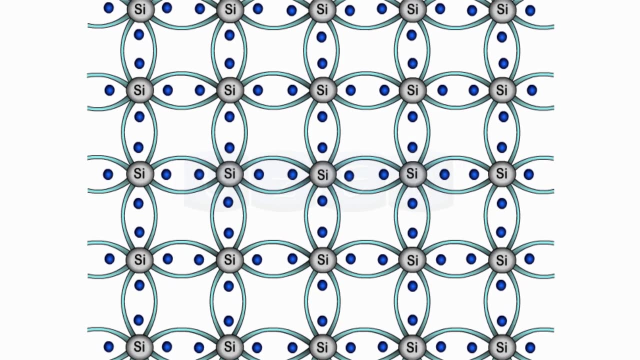 So we get a net negative charge due to this extra electron. Hence its name is n-type semiconductor. Common examples of n-type or pentavalent impurities are phosphorus, arsenic and antimony. When we add pentavalent impurities to an intrinsic semiconductor, 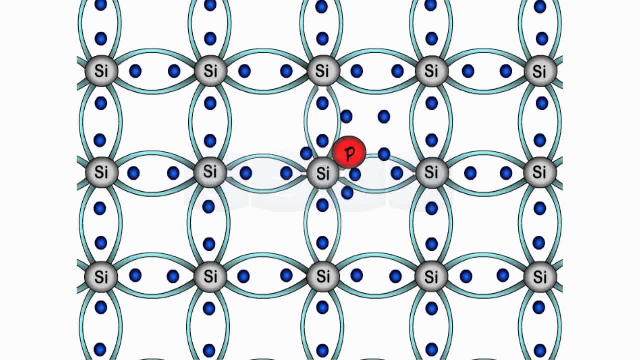 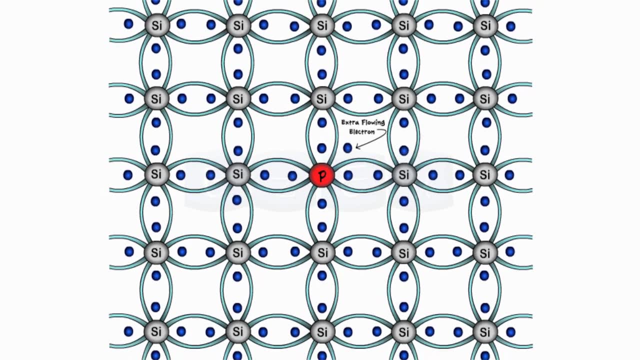 we observe that the phosphorus atom forms four bonds, with four silicon atoms fulfilling the needs of silicon, But even after that there remains one electron which does not form any bond and remains free. Hence, unlike the previous structures, here we get free electron readily available for conduction. 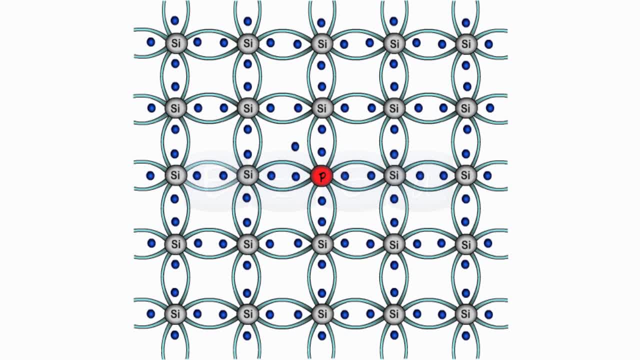 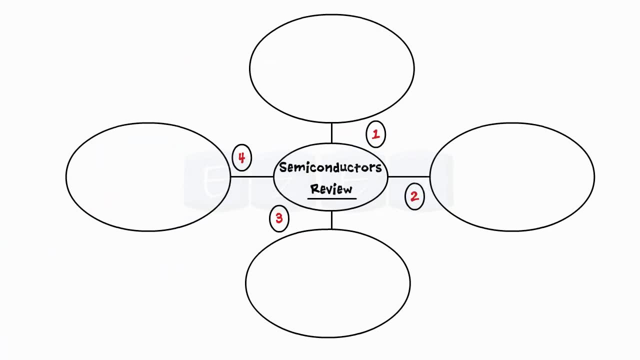 This electron rotates randomly around the phosphorus atom following a circular motion. In addition to this, the breaking of bonds, as seen in the intrinsic semiconductors, happens here as well. Now let's have a quick review of what we have learned in this lecture. 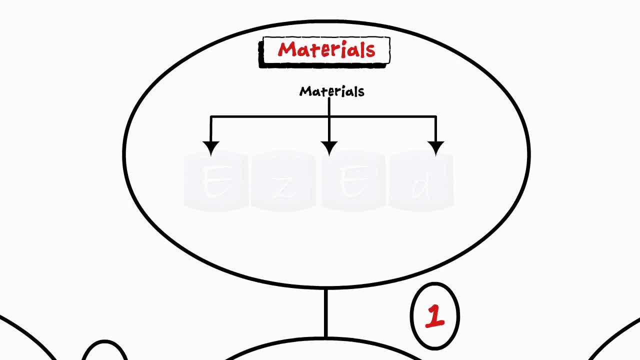 We categorize the materials into three main parts, such as conductors having excellent current carrying capacity, insulators having approximately zero current carrying capacity and semiconductors having current carrying capacity between conductors and insulators. Semiconductors are further classified into two main types. 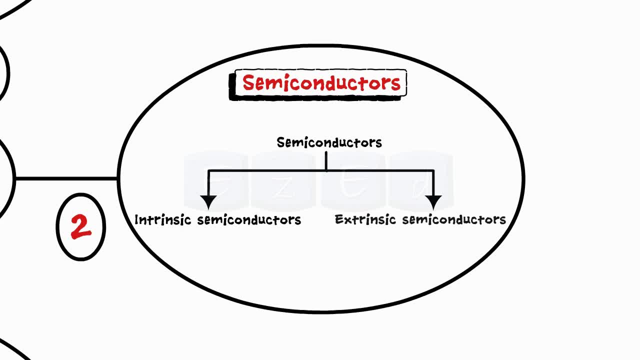 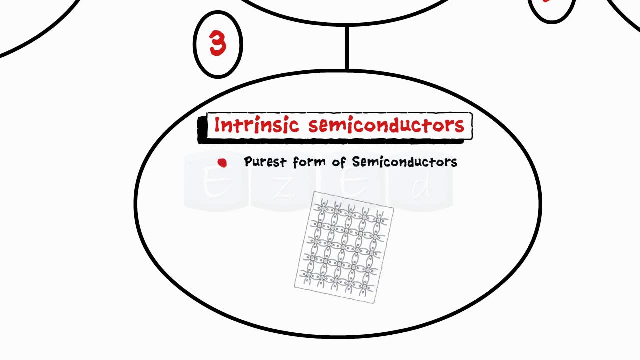 intrinsic semiconductors and extrinsic semiconductors. Intrinsic semiconductors are the purest form of semiconductors, having four electrons in the outermost orbit and made up of covalent bonding of silicon atoms with each other. 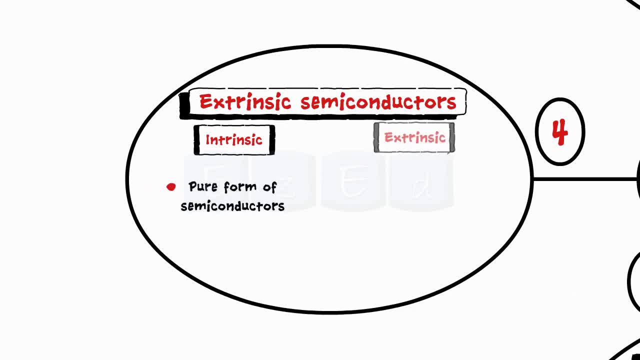 While intrinsic are the pure form of semiconductors, impurities need to be added to the intrinsic to improve their conductivity, and these semiconductors with impurities are called as extrinsic semiconductors. Extrinsic semiconductors are of two types. 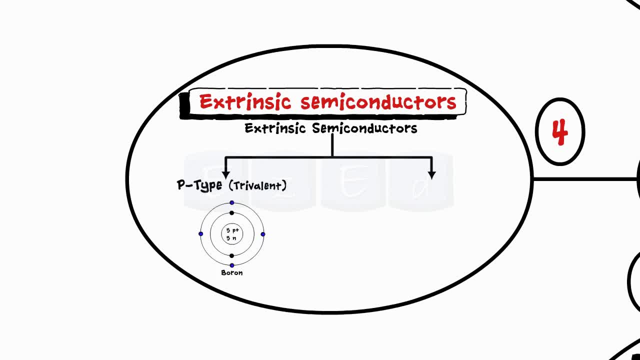 p-type, in which we add a trivalent impurity which has three electrons in its outermost orbit, and. n-type, in which we add a pentavalent impurity having five electrons in its outermost orbit. Addition of trivalent impurity creates a hole in the structure.